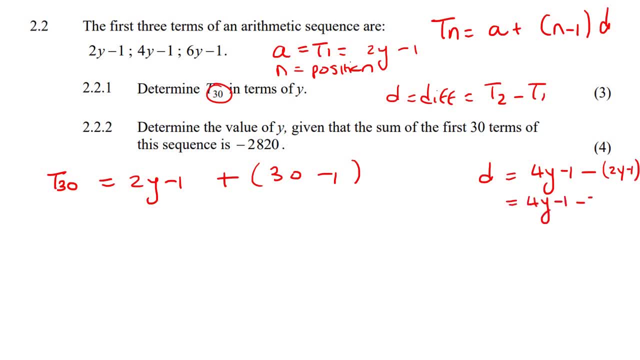 Okay, and so that's going to end up becoming 4y minus 1, minus 2y plus 1.. If any of you get this question wrong, it's probably because of that part over there, And then if we're to simplify that, 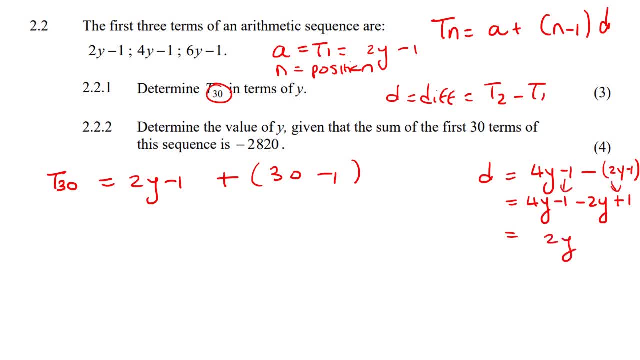 that'll just be 2y, because the minus 1 and the plus 1, they cancel out. So d is 2y, So we can just fill in 2y over there. Now we're going to just say that term 30,. 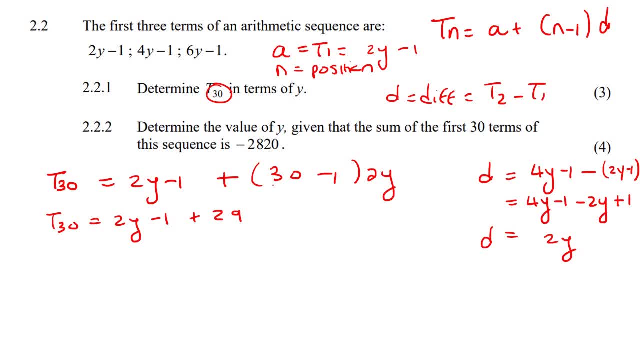 is equal to 2y minus 1, plus 29,, because that's what 30 minus 1 becomes times 2y, And so, if we carry on, we're going to end up with 2y minus 1, plus 58y, And so term 30 is going to end up being. 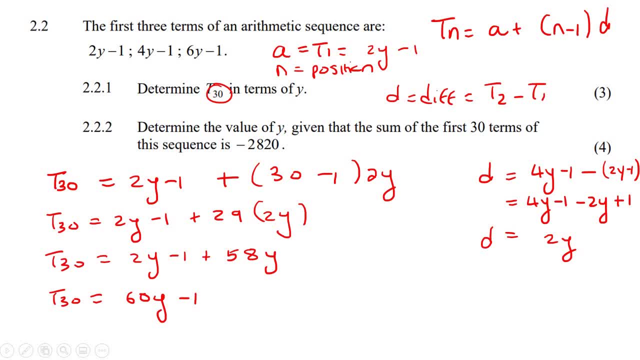 60y minus 1.. 60y minus 1.. The next question says: determine the value of y if the sum of the first 30 terms is minus 2820.. All right, so here's the sum formula of an arithmetic pattern. So let's go fill this all in. 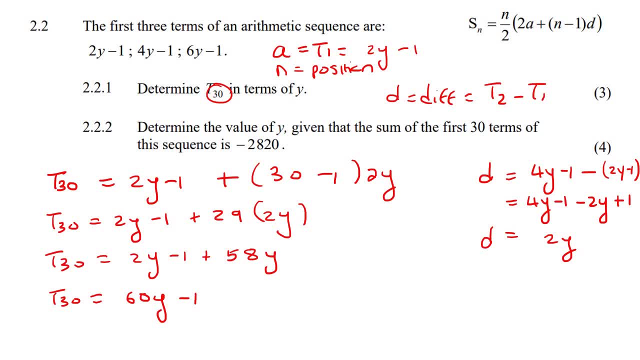 So they tell us that the sum of the first 30 terms- okay so- is minus 2820.. So we can say, we can say minus 2000,. let's give us a bit more space: minus 2820,. 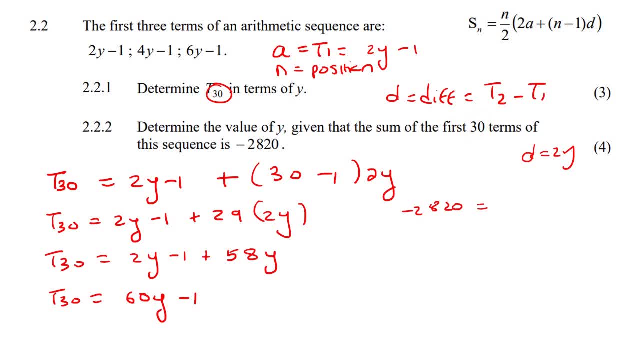 equals to n. Now n is the number of terms that they want us to use. They said the first, 30.. Now a is term 1,, which is still going to be 2y minus 1,, plus how many terms, 30.. 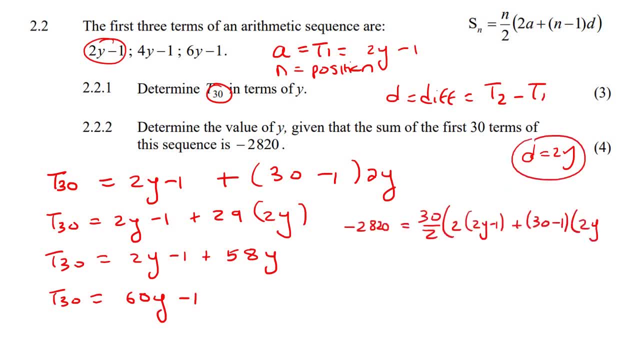 And then the common difference from earlier we said, was we calculated it as 2y, And so let's go simplify this now. So 30 divided by 2 is 15.. I'm then going to multiply that 2 into that bracket. 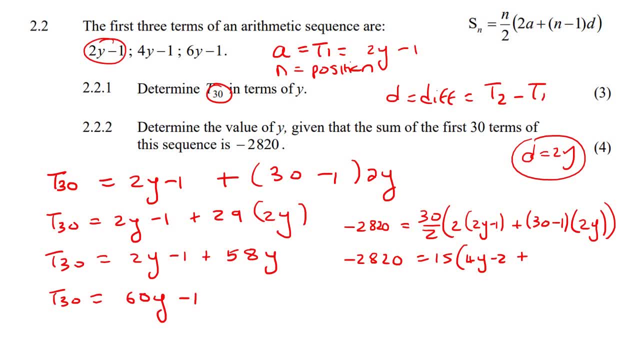 And then I know that this part just becomes 58y, because it's 29 times 2, is 58. And then there's that y, And then we can just simplify a little bit more by saying 15.. And then 4y plus 58y is 62y minus 2. And I'm going to multiply. oh, there's different ways.